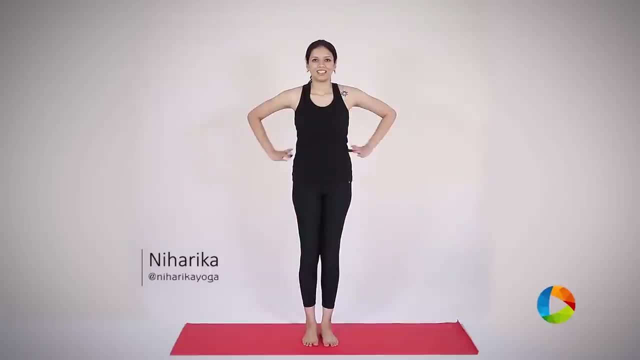 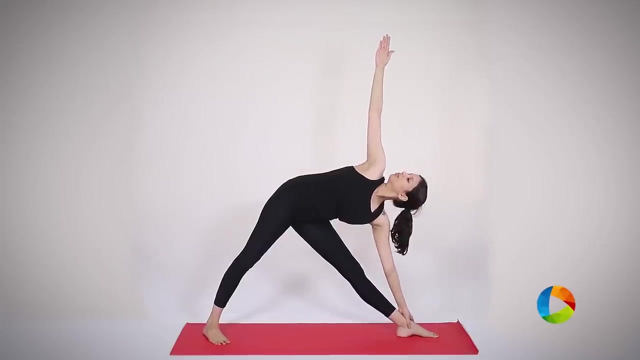 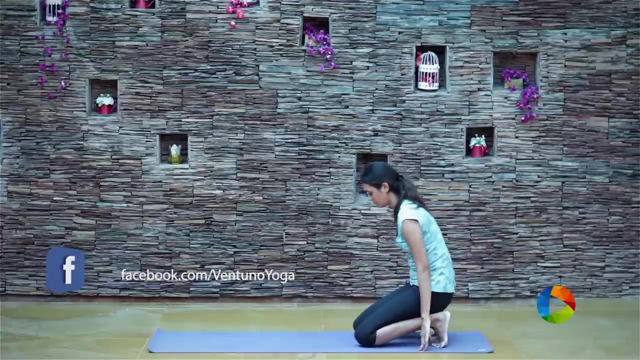 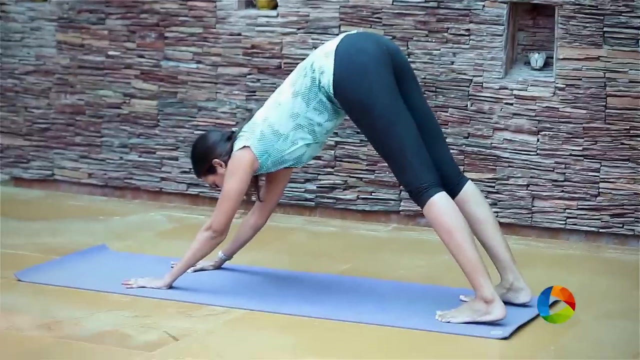 Inhale, Tadasana, Exhale, arms down and up. And now just try to do a balancing on your disc. Bring your knees down to the mat and fingers wide and nice and spread, Inhale. as you exhale, lift your knees and hips and send it back to the sky. And once you're ready, 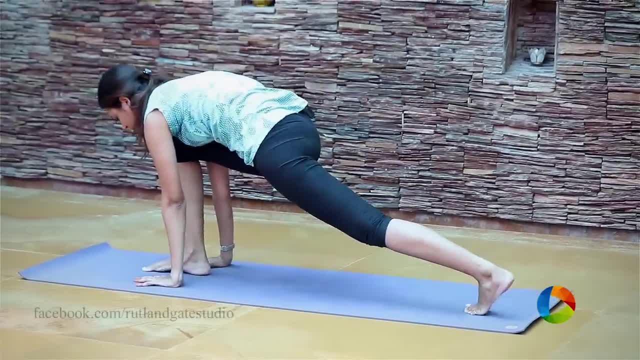 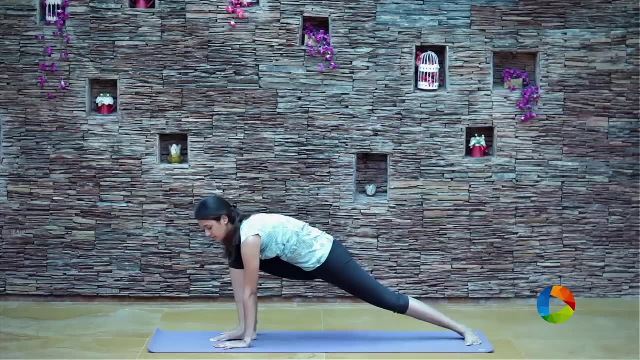 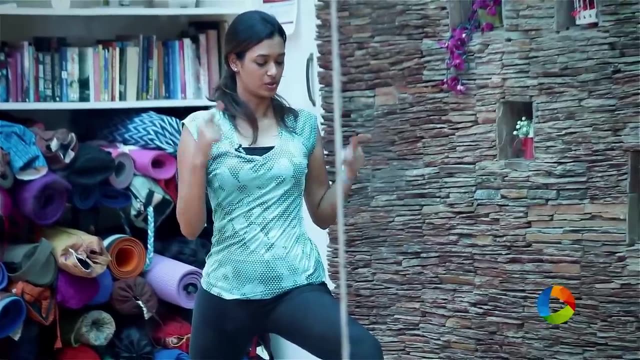 as you inhale, lift your right leg all the way forward and bring it right in between your palms, And the next step is to pivot your back foot to the mat, which is going to prevent you from falling down into posture. So from here, as you inhale, push yourself all the way up, bring your torso all the way towards your knees. 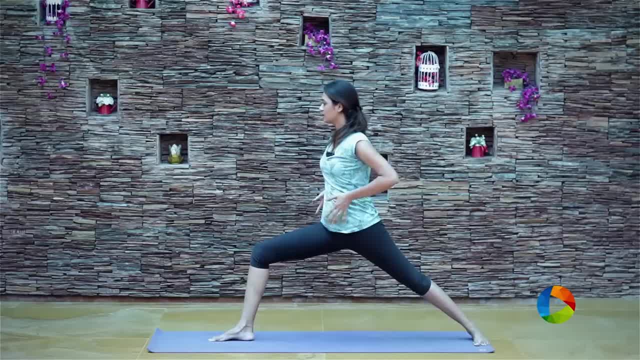 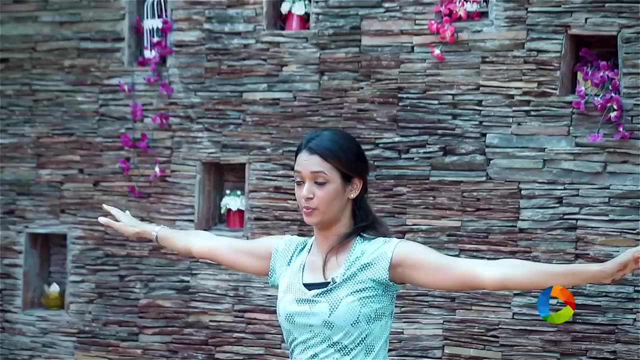 From here. once you're ready, maintain the lower body position And, as you inhale, bring both your arms all the way up and stay here for a couple of deep breaths. For number two, just keep your breath really normal and bring your body away from your knee. 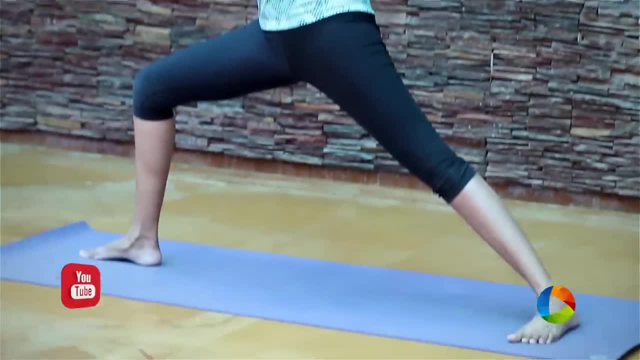 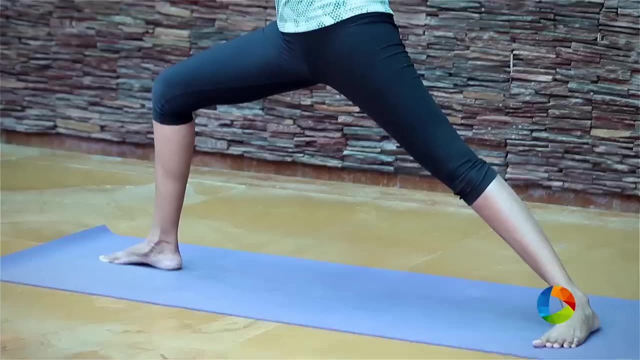 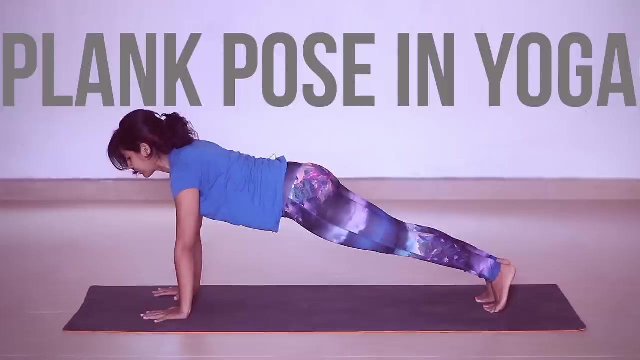 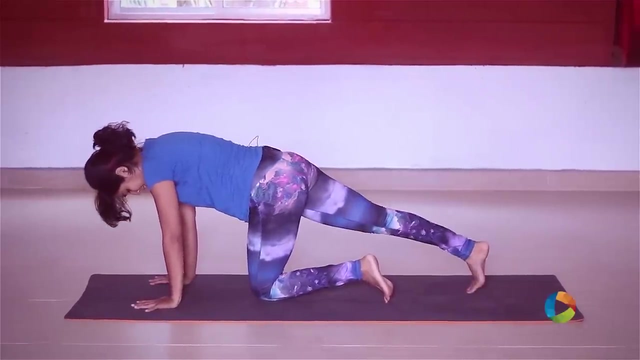 and still maintaining the knee position and the alignment, and stay here for a couple of deep breaths, For five, four, three, two, one Come to your mat, You bring your hands underneath your shoulders and extend your leg till your toes touch the ground. 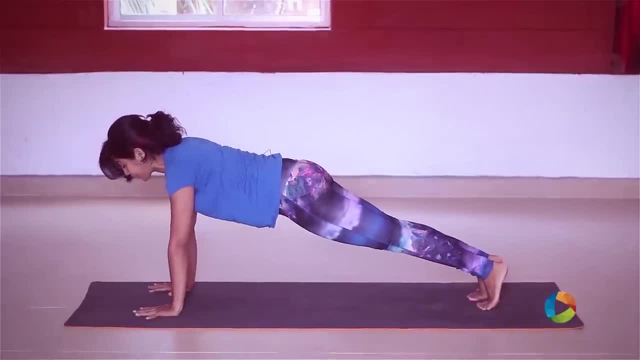 Then the opposite one. So always keep the body in a straight line, Because this is kind of Hard- people will have the tendency to do this- or drop your hips. That's really bad because you'll hurt your lower back. So always pull through your belly and make sure the body is in a straight line. 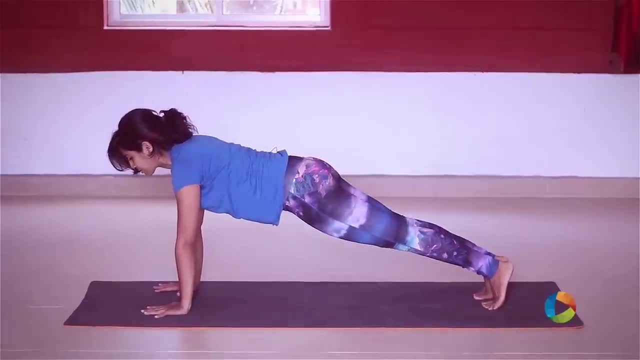 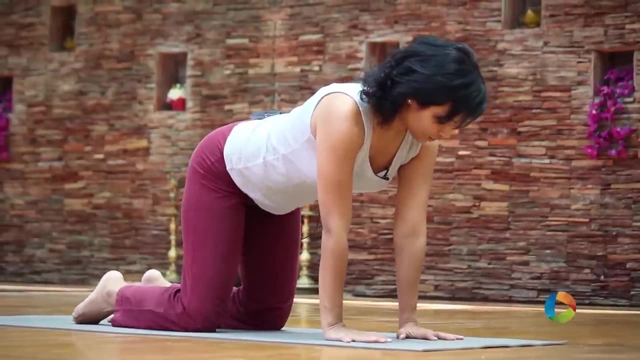 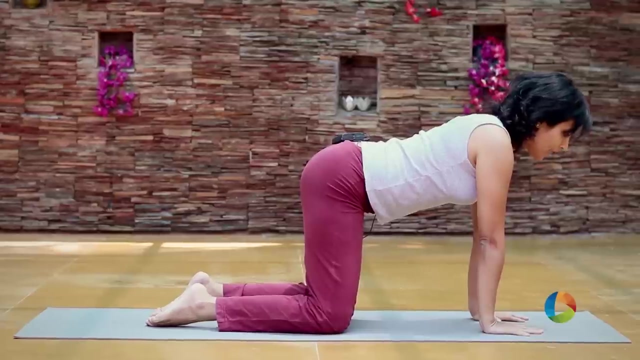 Roll the shoulders and keep the body really nice and long and engage your thigh muscles. Keep the wrist directly under the shoulders, the knees in line with the palms directly under the hip. The movement is only in the back and not in the limbs. 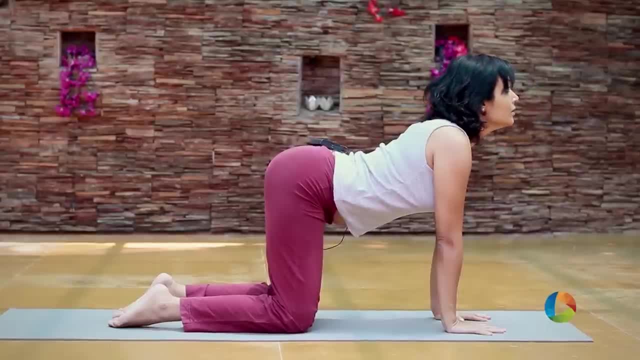 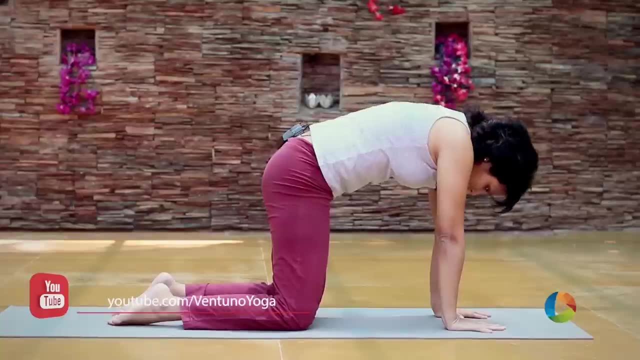 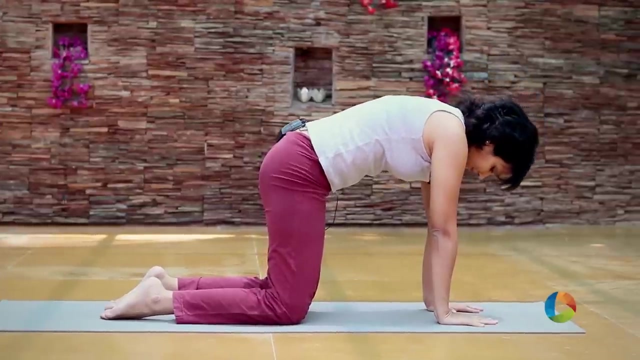 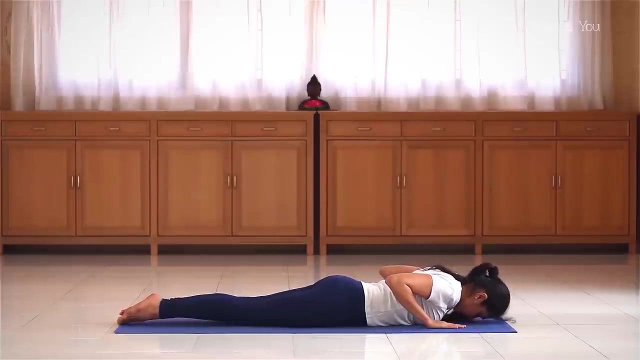 As you inhale, you drop the back down the head up. Exhale. you arch your back up, Look at your knees. Inhale- Exhale. Move the palms just beneath the shoulders- Inhale- head up.